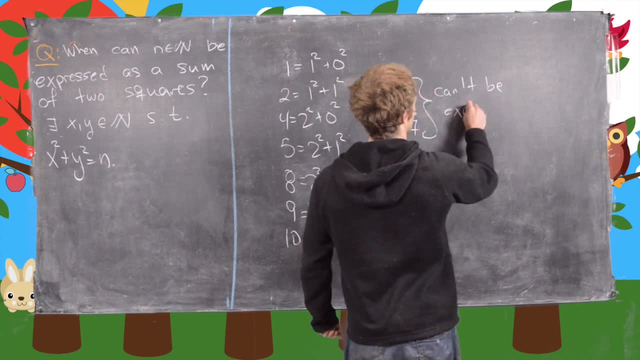 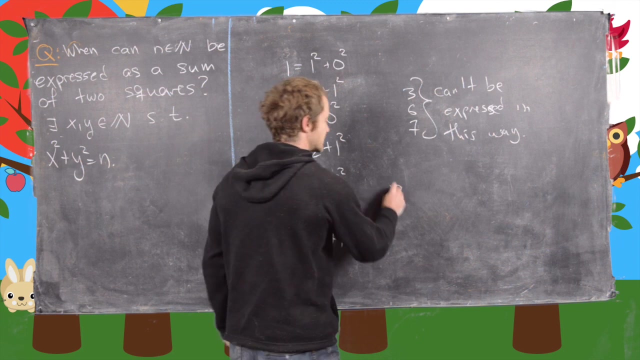 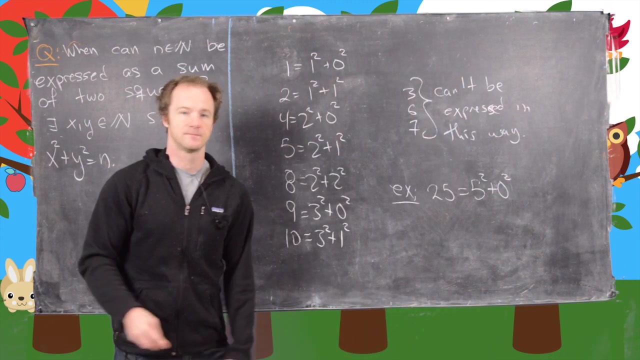 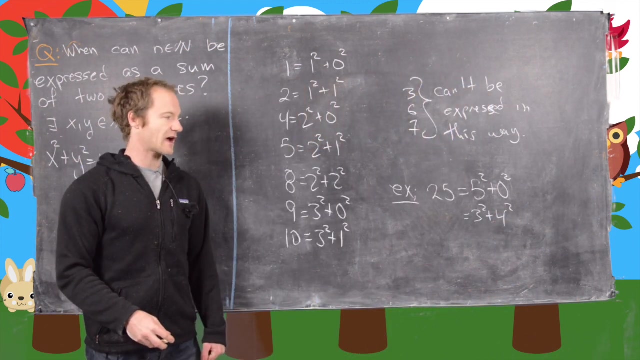 can't be expressed in this way, And in fact some integers can be expressed more than one way: as a sum of two squares. So let's look at a quick example, For example, of that notice that 25 is equal to 5 squared plus 0 squared, and also it's equal to 3 squared plus 4 squared, and in fact if you have a primitive Pythagorean triple, then that's automatically an example of a number that can be expressed two ways: as the sum of two squares. 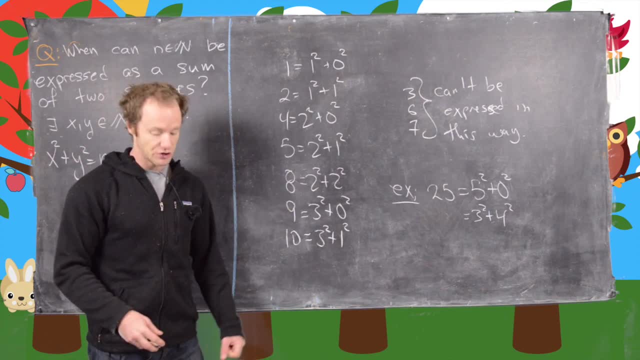 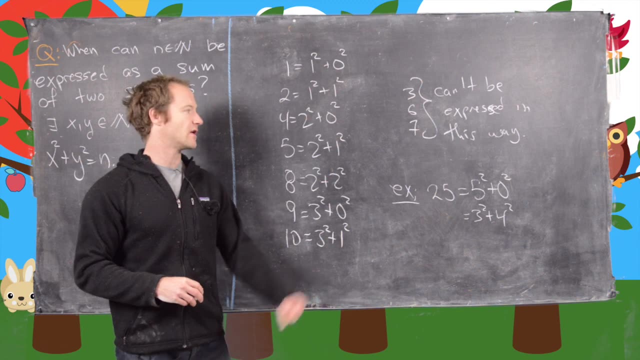 So I'll let you think about the details for that. Okay, so I've got two little results involving our path towards answering this question that I want to do in the remaining part of the video. Okay, so I've got two little results involving our path towards answering this question that I want to do in the remaining part of the video. 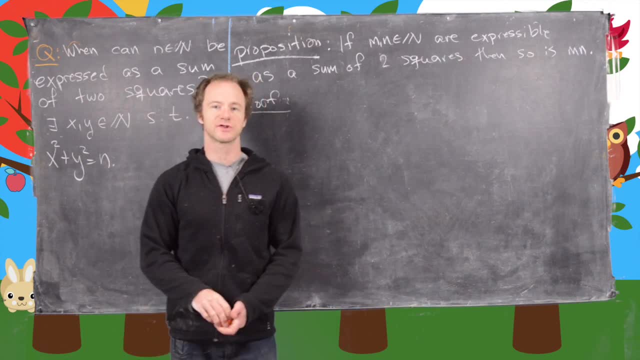 I'll clean up the board and then we'll get to the first one. Okay, the first little result we want to look at is the following: So if m and n are expressible as the sum of two squares, so is their product. 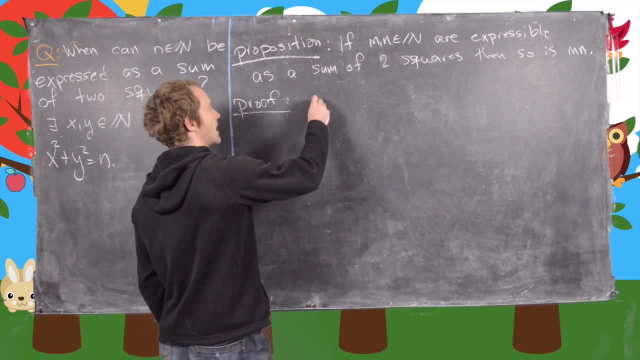 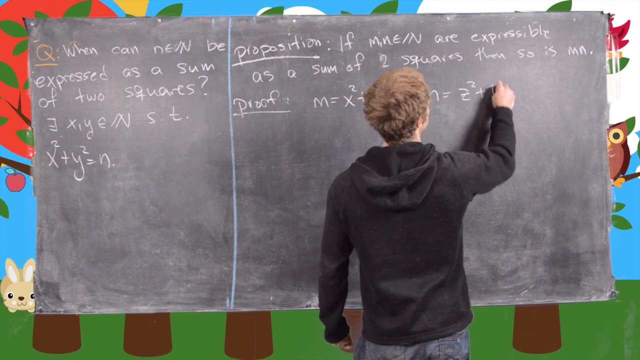 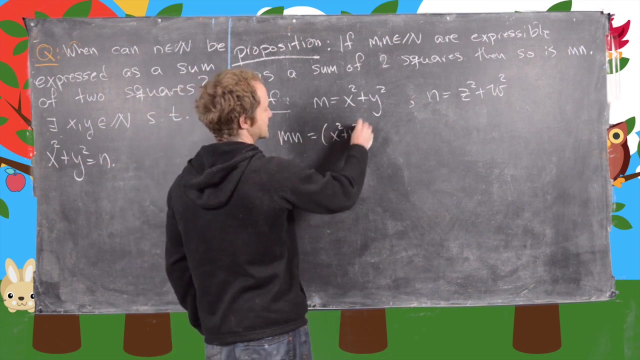 So this is a nice little result. So we're going to start off by writing the following: So we'll write: m equals x squared plus y squared. and we'll write: n equals z squared plus w squared, Okay, and then we'll take mn, So that's obviously x squared plus y squared times, z squared plus. 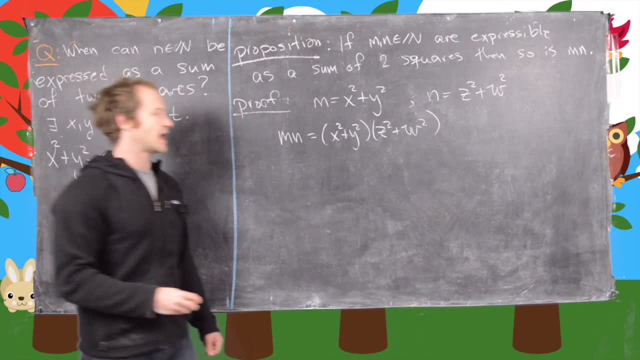 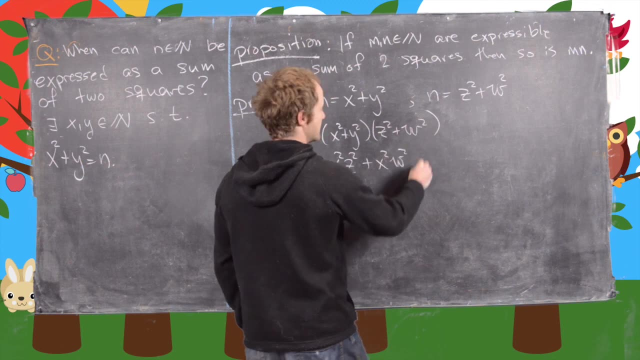 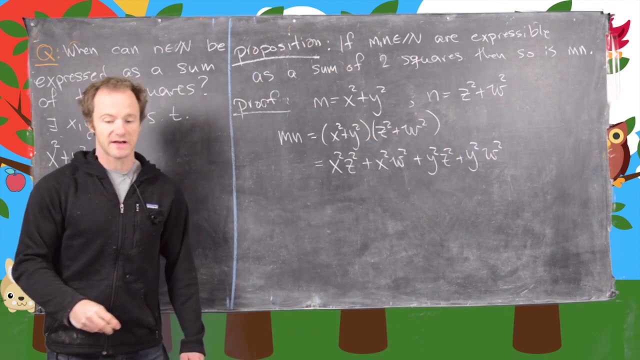 w squared, and We can FOIL that out. so we're going to get x squared z squared, plus x squared w squared, plus y squared z squared Plus y squared w squared. Okay, Now the next thing that we're going to do is add and subtract the same number. 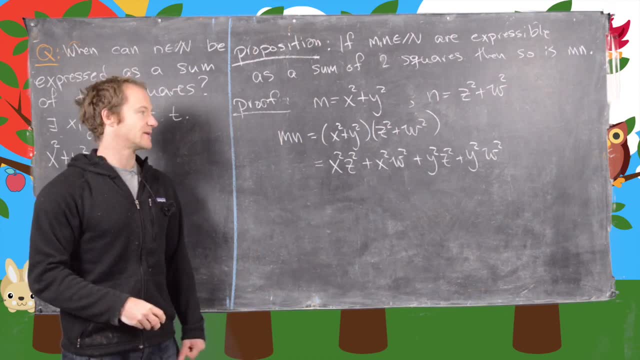 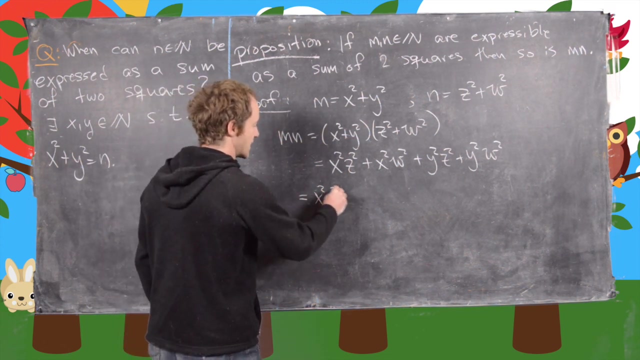 so we're going to add and subtract 2 x times y times, z times w, and then we're going to rearrange this in a way so that so that it factors into 2 binomial squared. So let's see how that goes. So we're going to start off by writing this: x squared, z squared. 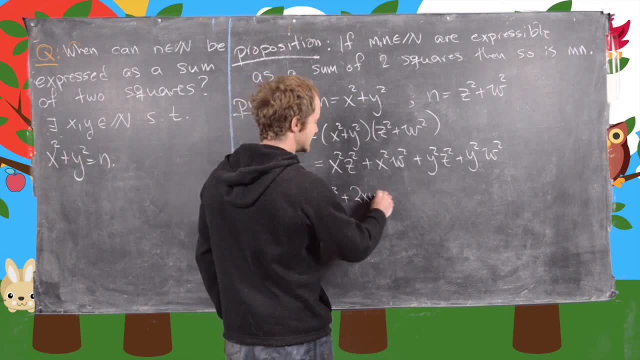 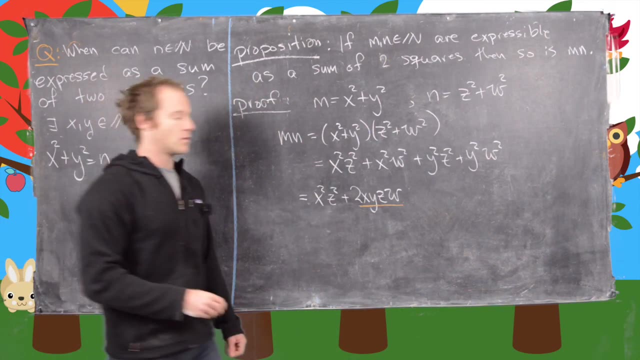 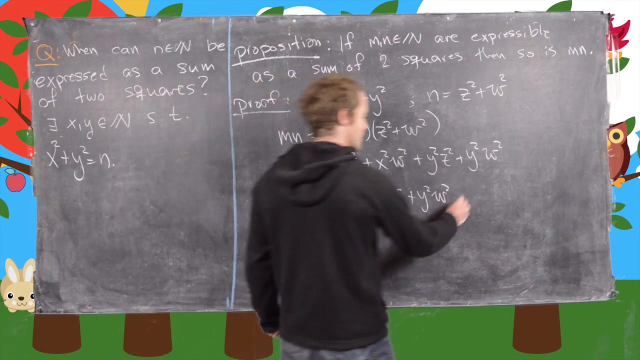 and now we're going to add 2xyzw. So there, we've picked up an extra term for the time being, And then we're going to put plus y squared w squared here. So we're going to move that one over, And now we're going to have plus x squared w squared. 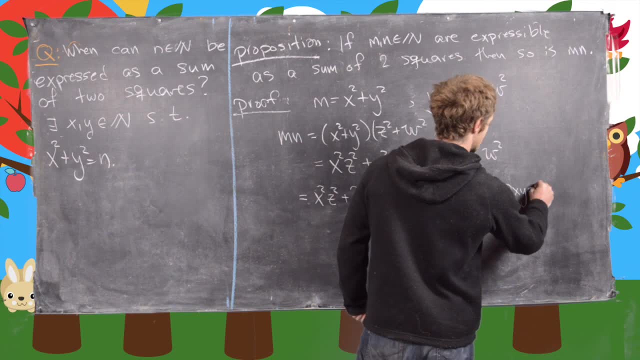 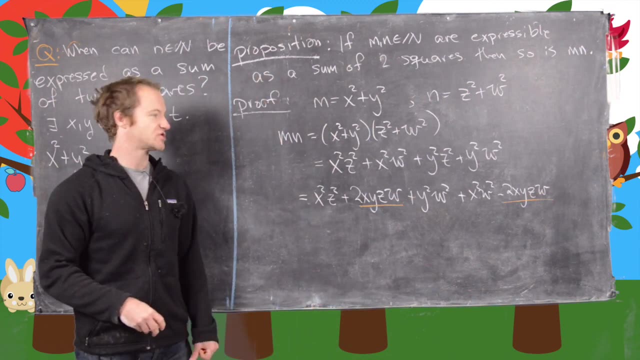 And now we're going to subtract this new term as well, So minus 2xyzw. So notice, we've just added and subtracted the same thing, so we haven't changed anything. And then we're going to have plus y squared, z squared. 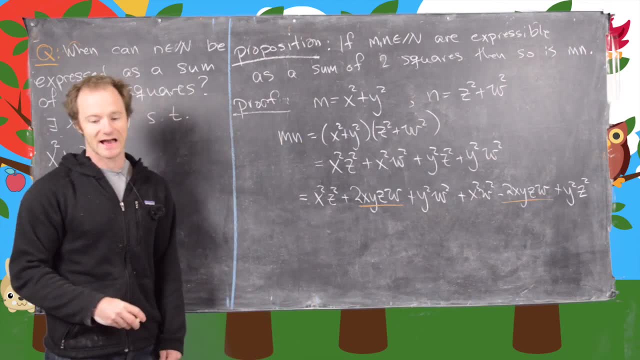 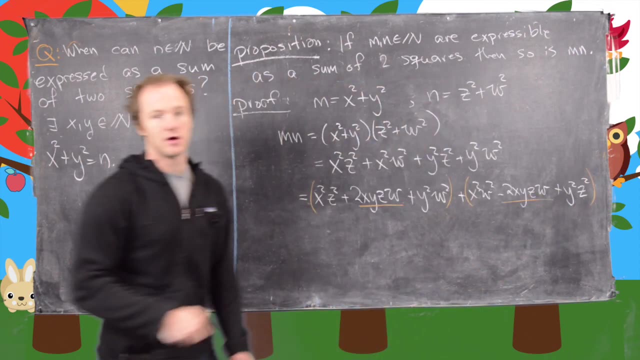 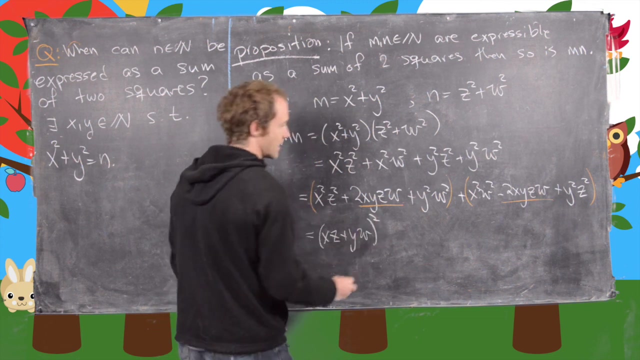 So this line is exactly equal to this line because we've just added 0.. But now We can do a little bit of grouping, So we can group these terms and these terms And then notice that they each factor. So this factors as xz plus yw squared. 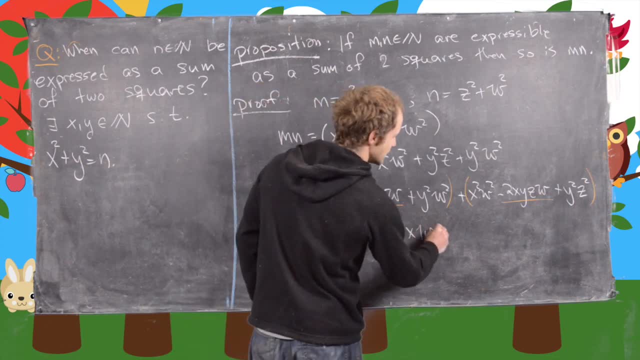 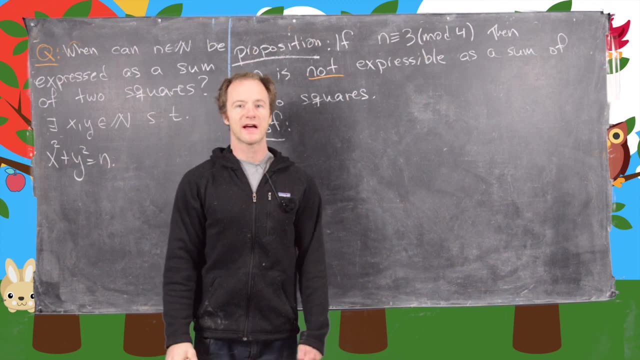 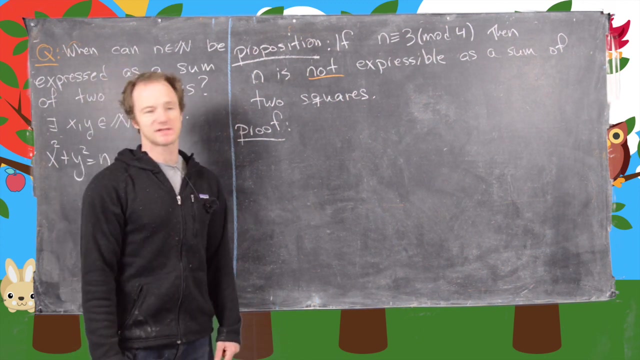 And then this one factors as xw minus yz squared. Okay, good, Okay. so next we want to look at this following little proposition: So if n is congruent to 3 mod 4, then n is not expressive. It's just not possible as a sum of two squares. 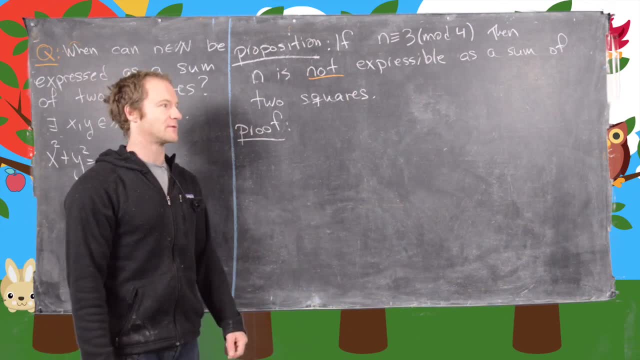 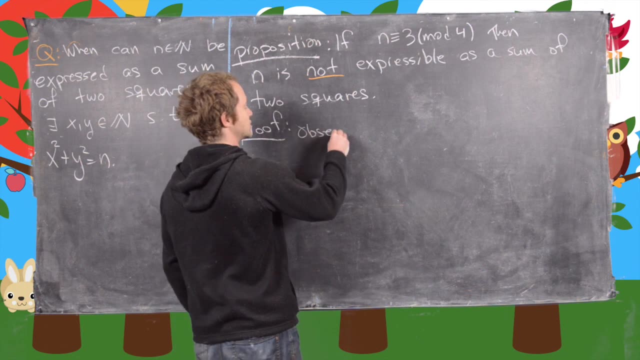 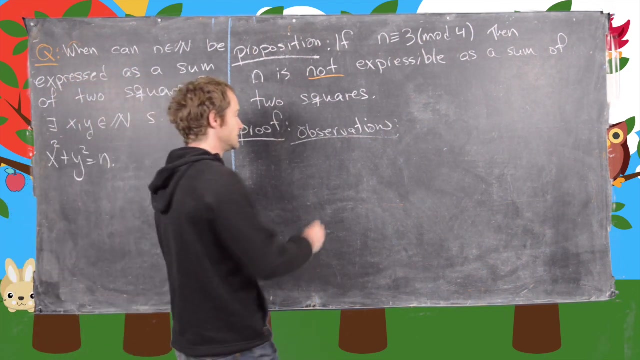 Okay, so this is actually something you've probably already seen in a homework problem or something like that before. It's just the dots weren't connected all of the way, And so let's start off with the following two observations, Which are easy to show, and I won't do that. 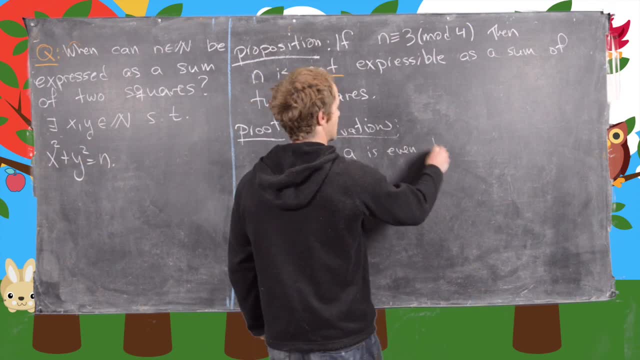 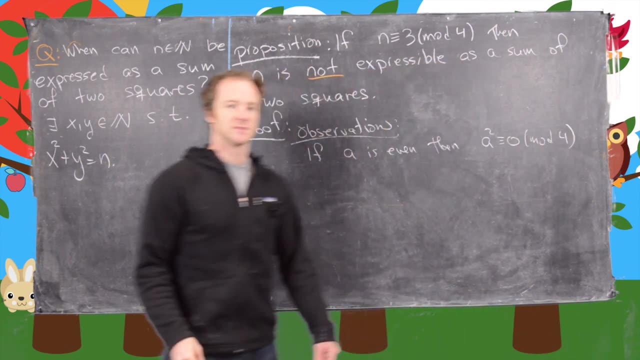 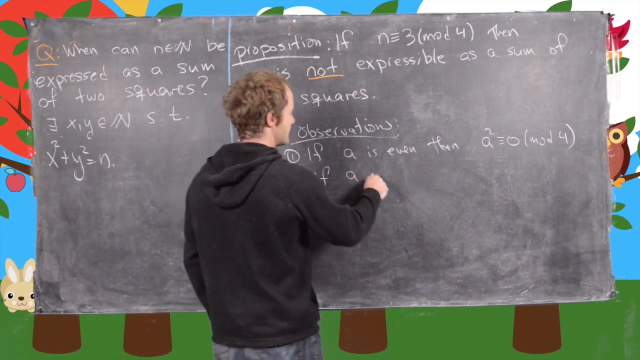 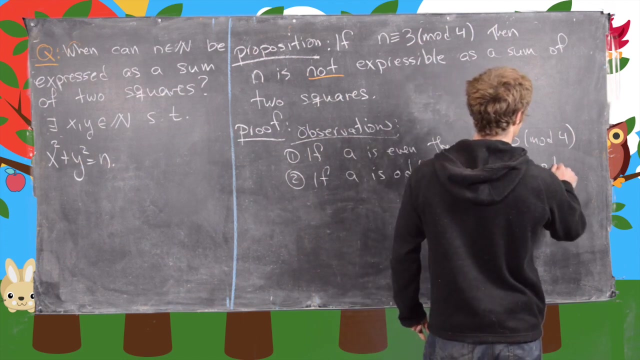 So if a is even, then a squared is congruent to 0 mod 4.. So that's like super easy to show Again. I'll skip that. And then the second observation is the following: If a is odd, then a squared is congruent to 1 mod 4.. 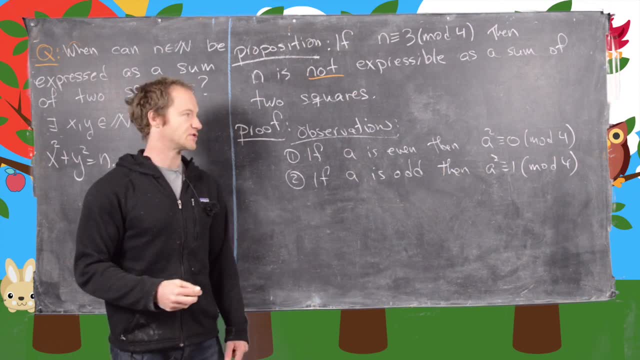 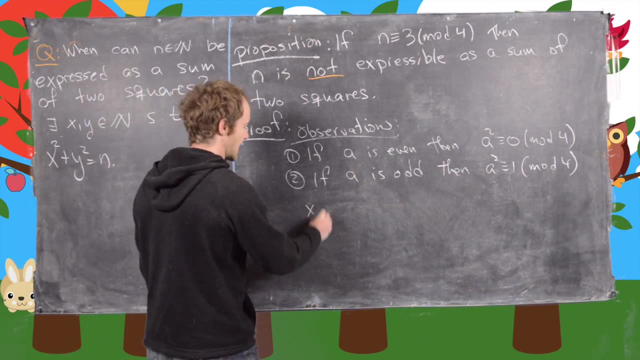 That essentially comes from the fact that 3 times 3 is 9, which is 1 mod 4.. Okay, now the next thing that we want to do is like look at this little chart. So let's look at a chart x- y. 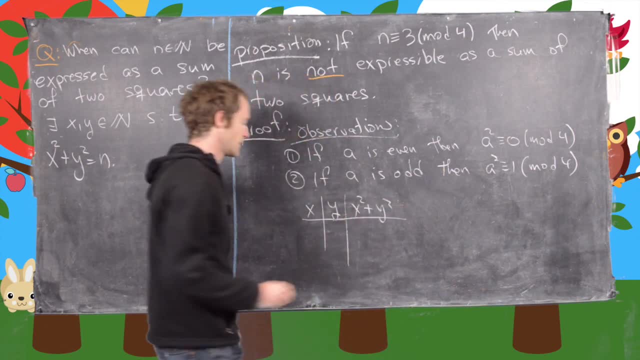 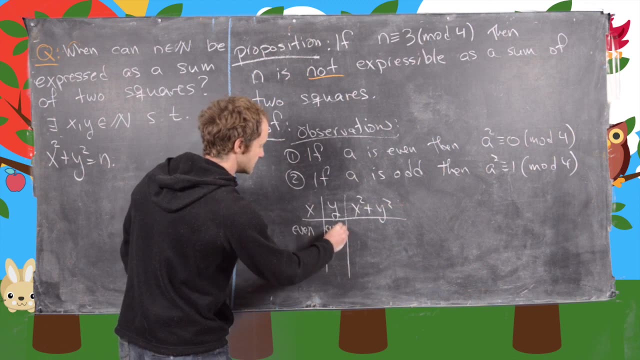 and then x squared plus y squared And notice that we have three big possibilities here. They could both be even, or they could both be odd, Or one could be odd and one could be even, And since x squared plus y squared is symmetric, 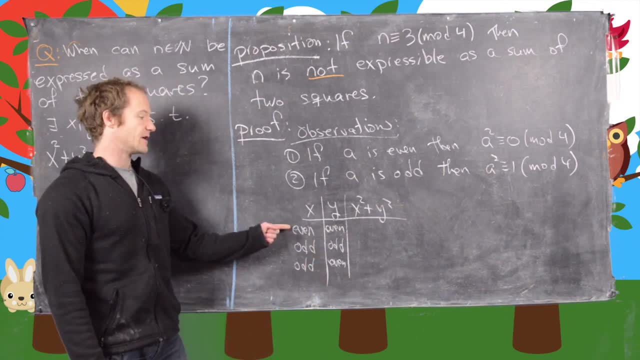 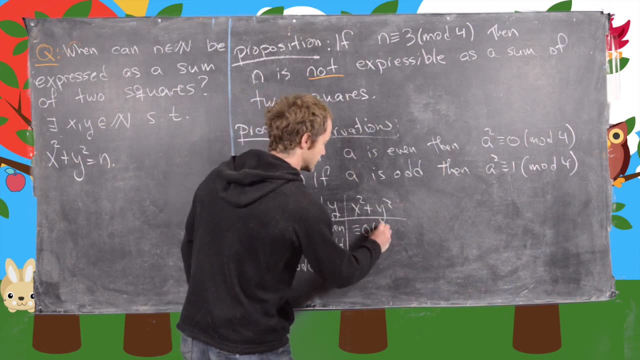 it doesn't really matter, We don't have to look at the other case. So now, if they're both, even, that means they're both congruent to 0 mod 4.. And so that means their sum is also congruent to 0 mod 4..